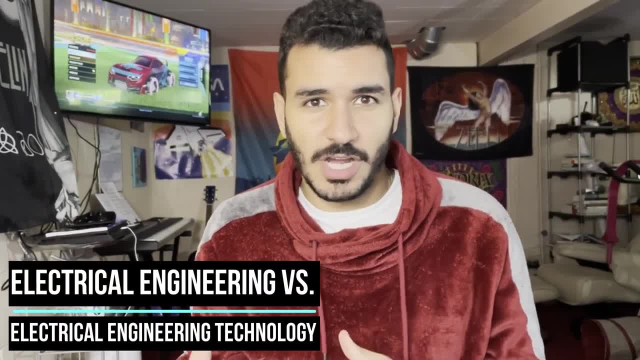 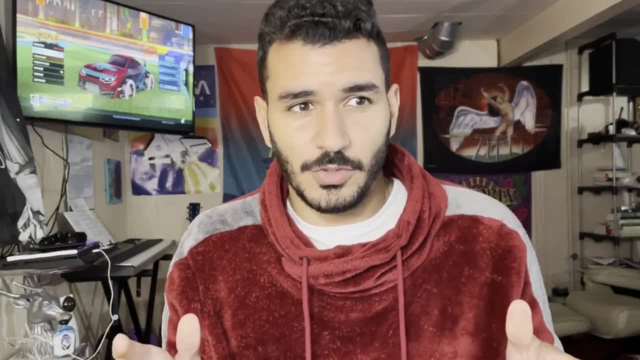 so electrical engineering and electrical engineering technology have more in common than you think, although there are big differences and you should be careful of these big differences. this video i'll tell you about these differences and help you decide which one is better for you, and i'll tell you why i chose electrical engineering over electrical engineering. 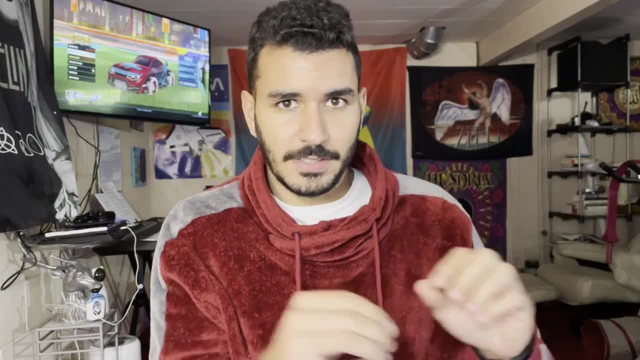 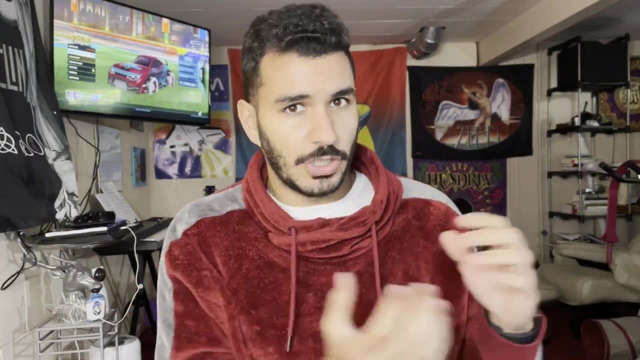 technology. there's two things i want to tackle here. one is the skill set and two is the societal perception, or like career path or like- i don't know- ease of getting hired in the job that you want. you may already know that electrical engineering involves more math and physics. 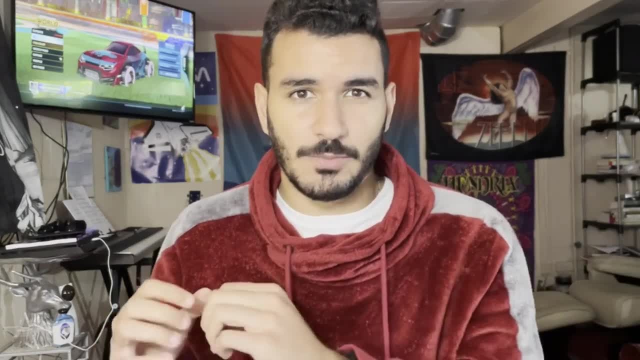 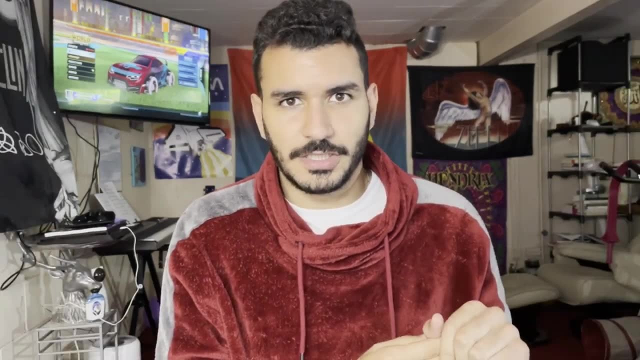 and theoretical conceptual design. where electrical engineering technology is more hands-on is about implementing and maintaining those electrical systems. from a skill set perspective i would say: only go the electrical engineering technology route if you're absolutely not interested at all in math and physics and you're not curious at all about the theory of. 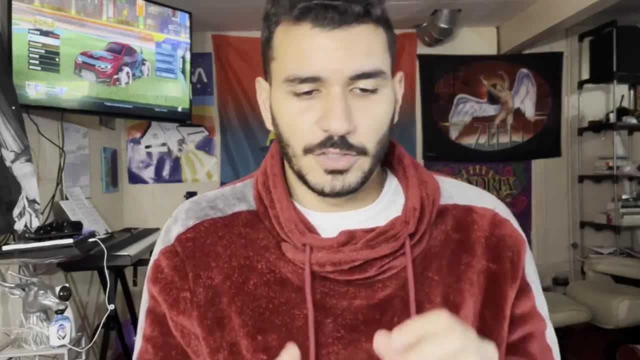 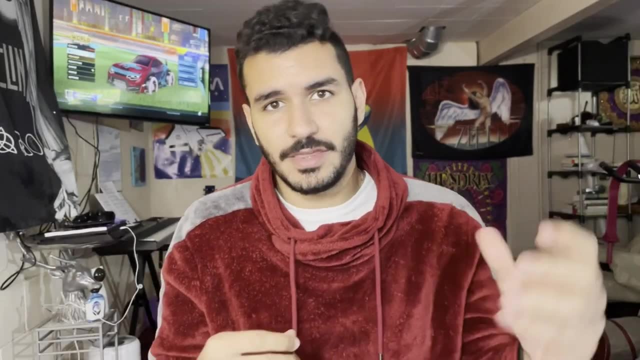 why electronic and electrical systems behave the way that they do. now, for an electrical engineering degree, you don't have to absolutely be in love with math and physics or with a theory, but you should be at least curious about why things behave the way that they do, because this curiosity is the 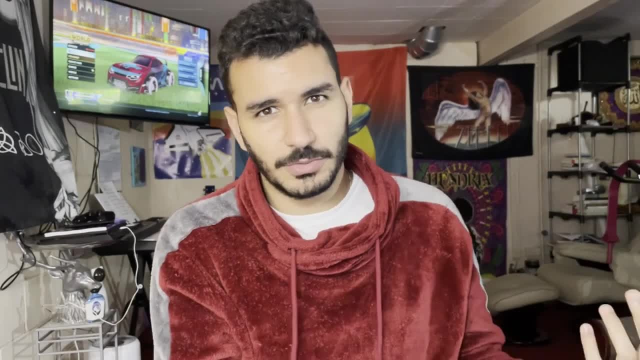 series of questions that you have to ask yourself when you're thinking about what you're going to do: current ingredient to design and research development, which are things that you only can really do with the electrical engineering degree. so if you're curious about why things behave, the 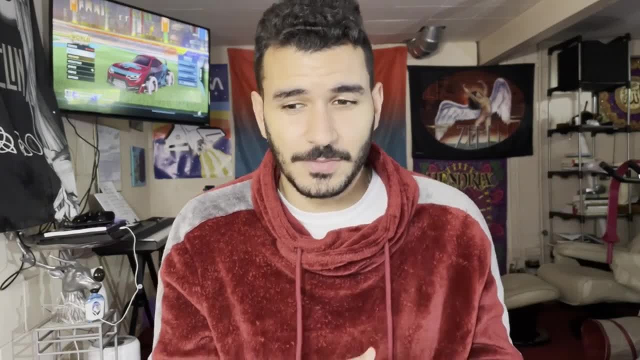 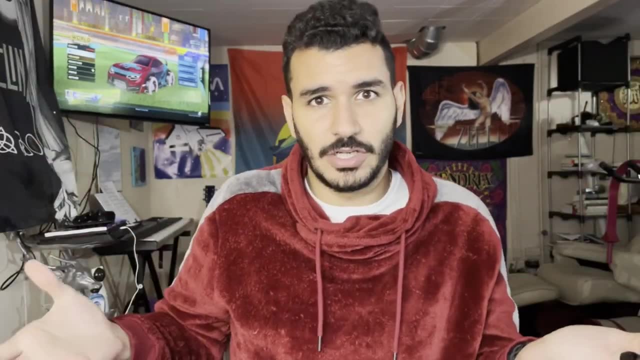 way that they do, especially like electronic and electromagnetic systems. i would say: definitely go for the electrical engineering degree and then go do some hands-on projects on the side, and that way you get both: you get theoretical knowledge and the hands-on knowledge. and that's actually what i did, because the reality is that with the electrical engineering technology degree you're 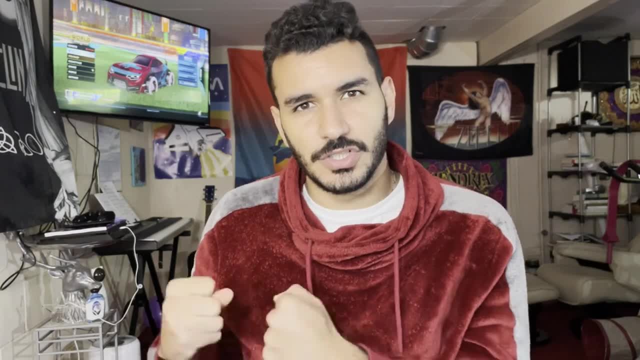 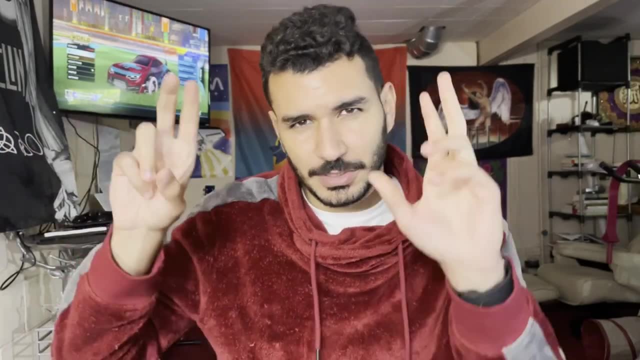 not really going to develop the deep understanding of maxwell equations or understand why things behave the way that they do. now, that takes care of the skill set. what about the career path? slash job. you're going to get slash. how are you going to be looked at like? will you be equally? 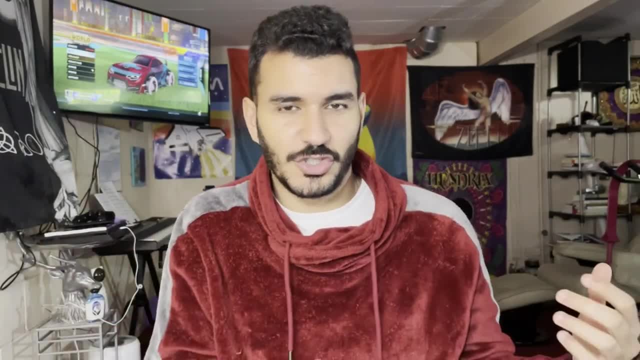 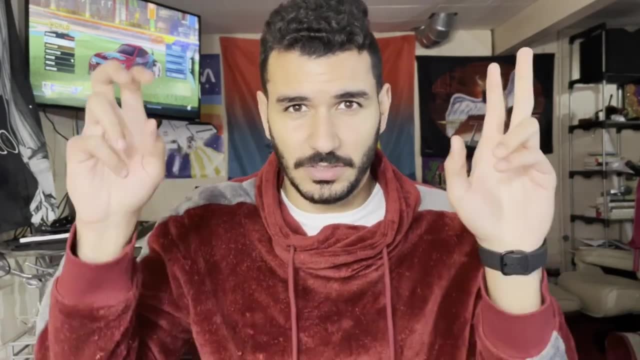 respected as an electrical engineering technologist rather than just an electrical engineer, and there's two ways to answer that. me personally, i don't care at all. i only look at people's skills. i don't really care, like what letters they have after their name or what degree they have. 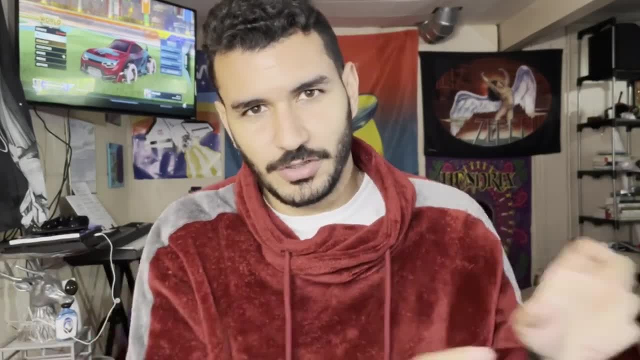 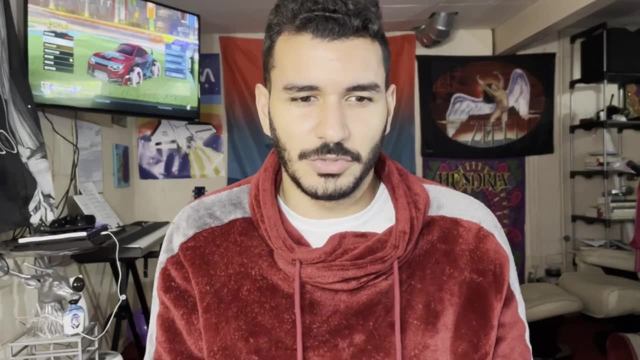 i really don't like labels, and just because you tell me you did the technology degree rather than electrical engineering degree, that does not signal to me: oh, this guy is dumb or can't do math, but rather it tells me: oh, this guy is probably self-aware and realized they don't like math. 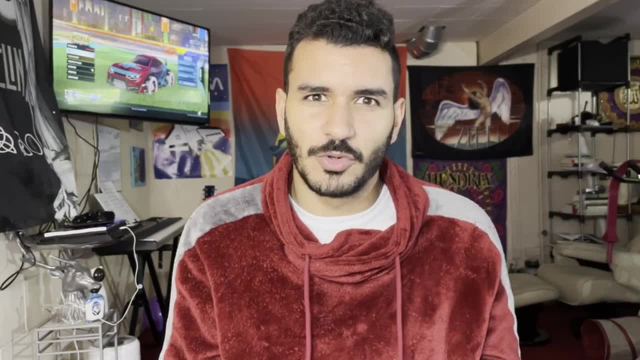 and physics and they still like technology, and they don't like math and they don't like technology. so they chose to do something that's a bit more hands-on and i totally respect that. however, from a general societal perspective, i know that society as a whole cares about labels more. 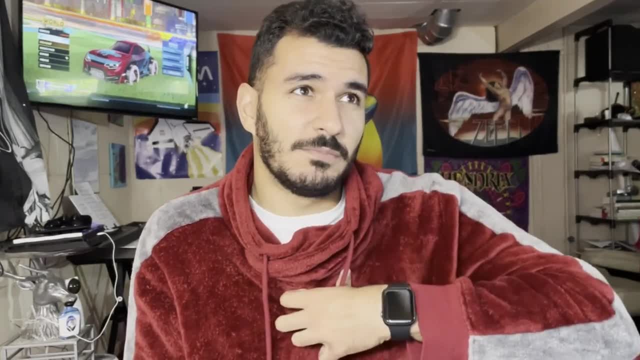 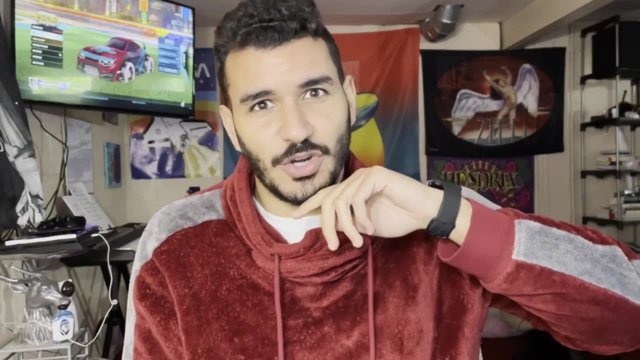 than i do. i mean, i don't know, because i've never experienced that myself. my guess my gut feeling tells me that there are people out there that who are probably not ill-intentioned, they're just conditioned to think that way, that may look down on that degree and may think: oh, you're not. 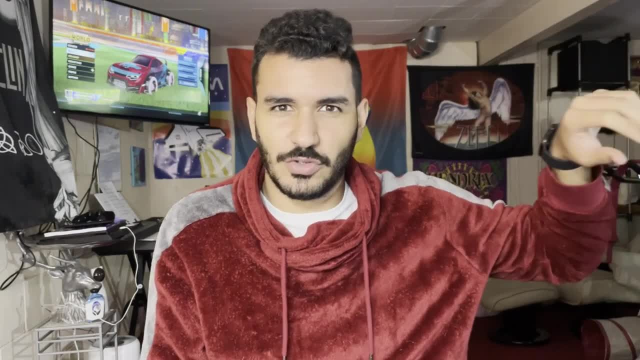 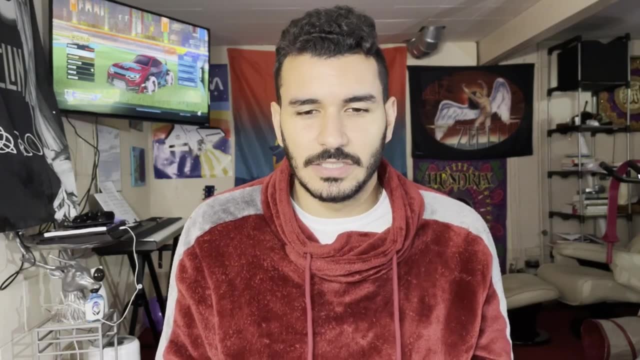 a real engineer or like: oh you're not, you've not done the theory, so you're only as good as technician. you're not a real problem solver, and for that it's very important for you to understand what you like and what you want and and to think critically for yourself, because you can't let 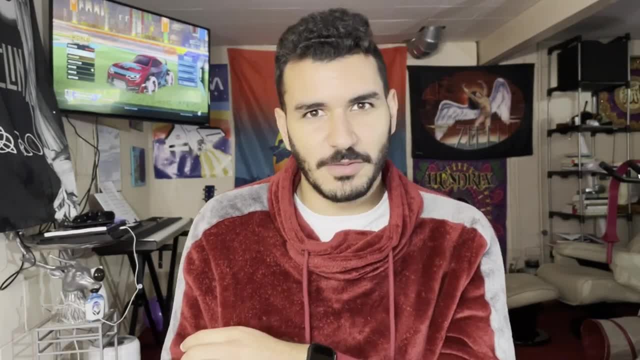 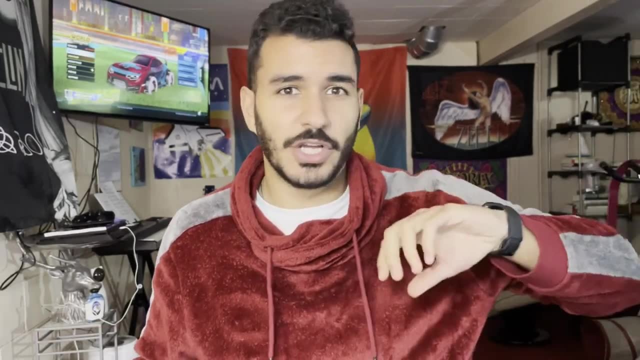 other people's or societal perception dictate whether you go for something or not. if you are absolutely only interested in the hands-on stuff, you don't care about the math and physics at all. you don't care about the theory. it does not excite you. you're not curious about why electric fields. 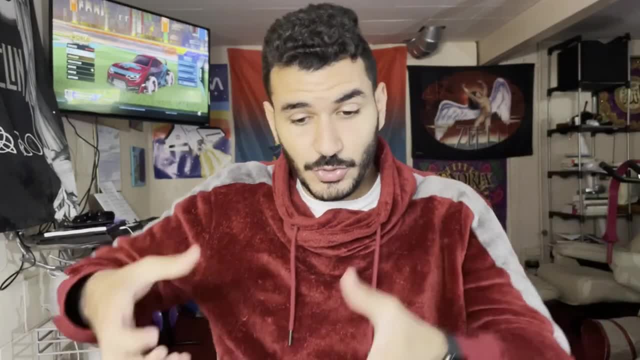 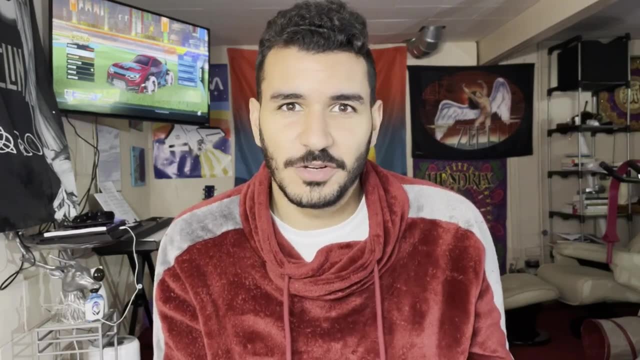 when changing induced magnetic fields, like if that sounds horrifying to you but you still like to grab the technology and take it apart and fix it and build things and implement things and systems. then who cares whether, like someone thinks, oh, you're not a real engineer, well, like that's, that's their own, that's their own problem, not yours. and again this kind of mantra. 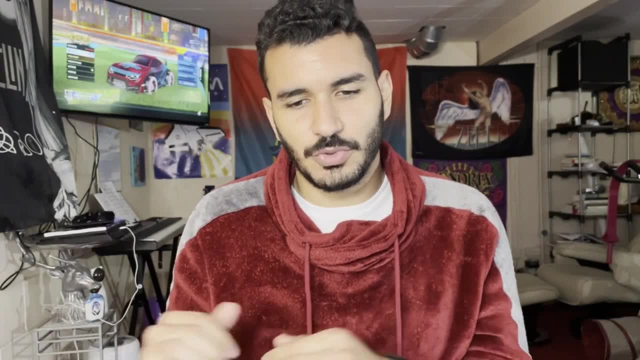 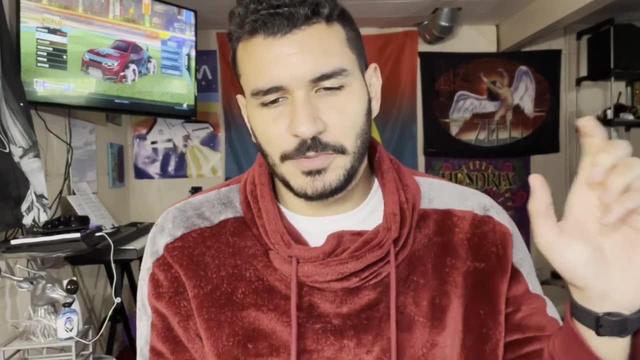 i have on this channel is: just be so good that they can't ignore you. just be really good at what you do that you don't really run into these people and if you do, you don't even care because you have opportunities and you have a career path set for you and, generally speaking, anybody who 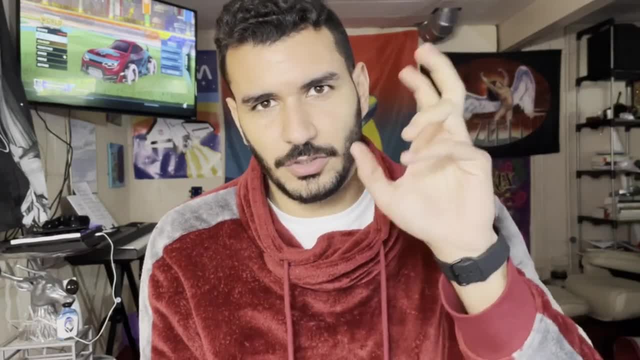 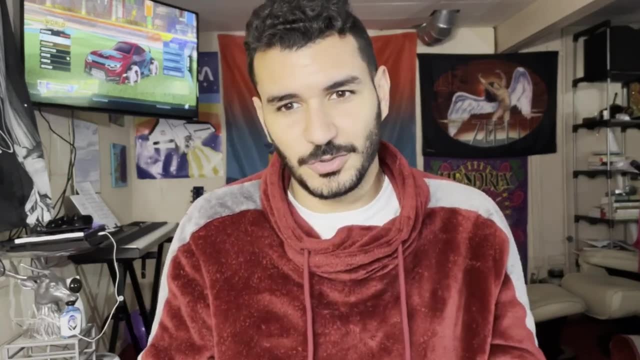 is conscious and has deep understanding of the importance of skill set rather than degree or label, will not really give you that kind of issue. however, the reality is that if you want more value for your book and if you really want to be hardcore in electrical engineering, you would probably do. 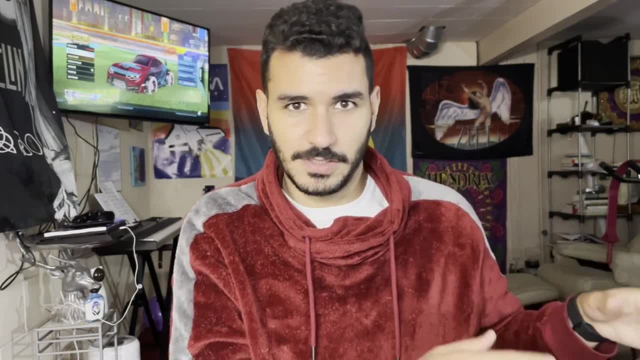 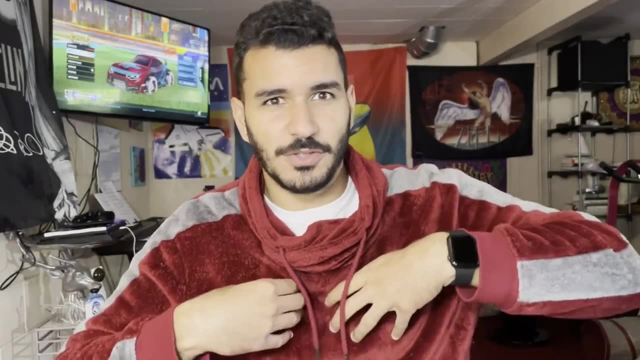 the electrical engineering degree. go through the theory, go through the physics- one, two, three courses and do the hands-on stuff on the side. that would make you like a more complete electrical engineer. but again, that's just me, that's my personal belief and that's what i. 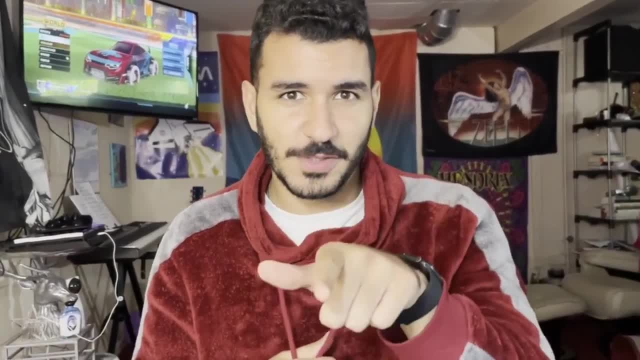 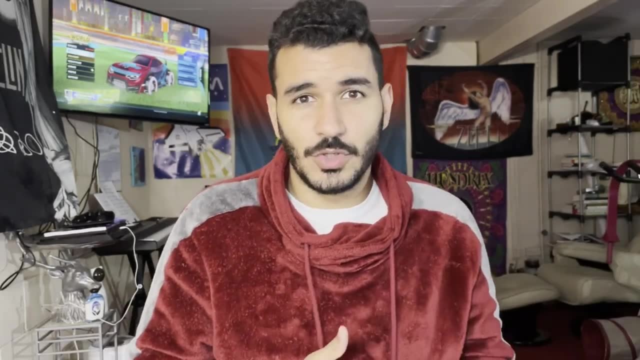 chose to do, and that's one guy. so you should do some thinking on your own, decide what's best for you. i will also leave a note that if you're not sure about what to do, you probably should not limit yourself to one area over the other, because, who knows, maybe a few years down the line you'll 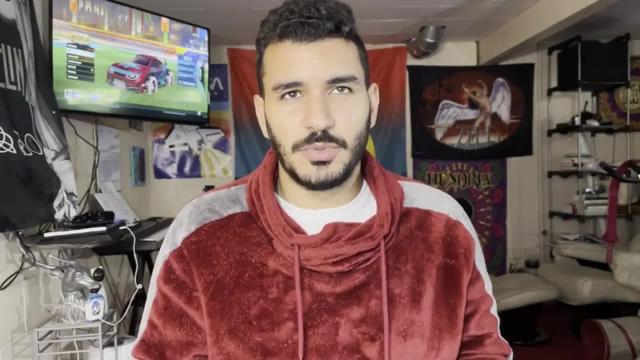 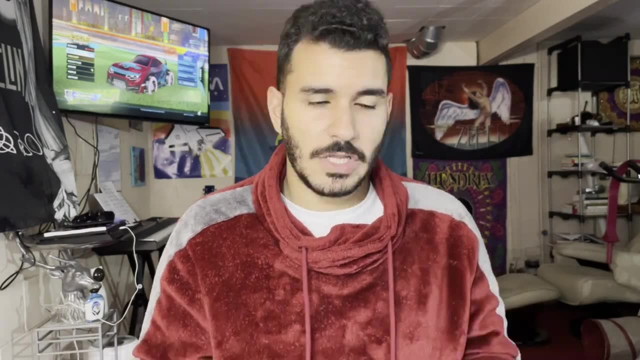 be a lot more interested in research and innovation and you probably want to keep your doors open. so you might go for the thing that's harder initially but keeps your options open. but again, that's just i think about things. so i personally am curious about the theory and this is exactly why i chose. 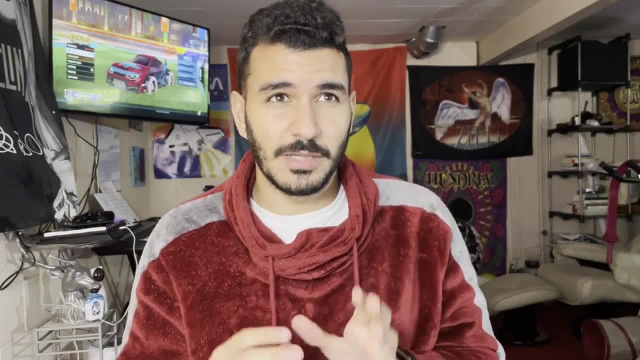 to study electrical engineering. in fact, there are 17 reasons that i was able to come up with on why i chose electrical engineering and why you should probably choose electrical engineering, and i made a video about it, so you should watch it over here.